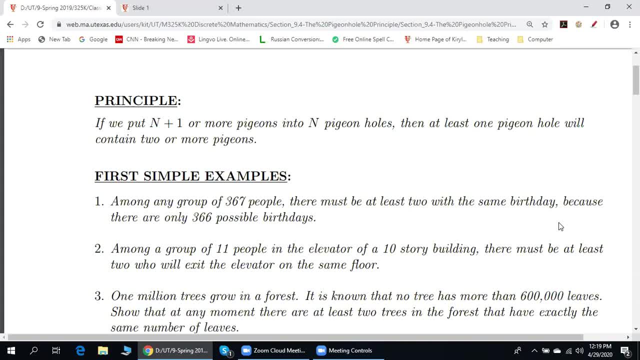 there will be a pigeonhole that contains at least two pigeons. Next, among a group of 11 people in the elevator of a 10-story building, there must be at least two who will exit the elevator on the same floor. What are pigeons? What are pigeonholes? 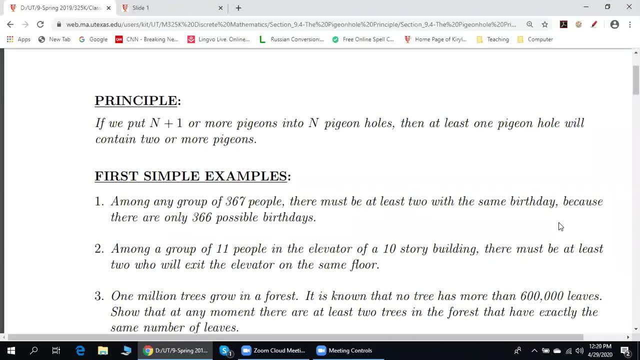 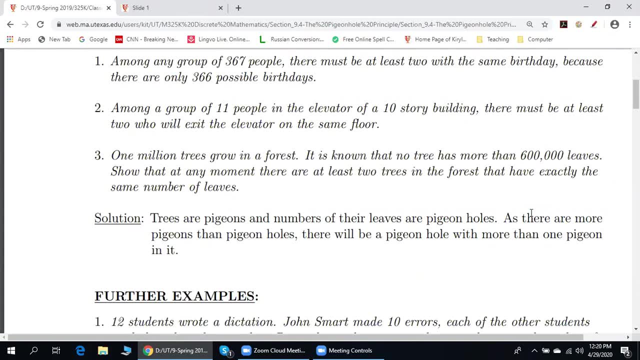 People are pigeons. The story are the pigeonholes. Yes, Okay, Example number three: One million trees grow in a forest. It is known that no tree has more than 600,000 leaves. Show that at any moment there are at least two trees in the forest. 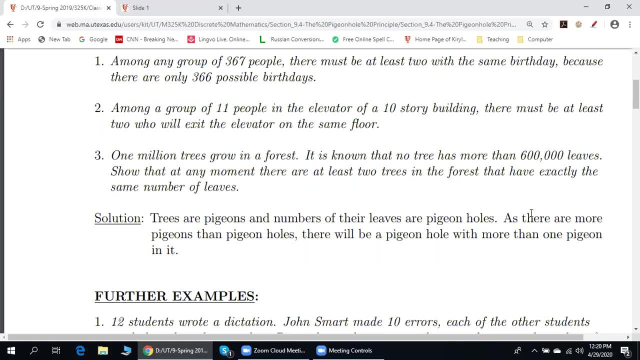 that have exactly the same number of leaves. Trees are pigeons. We have one million pigeons And the number of leaves are pigeonholes. So, since there are more pigeons than pigeonholes, there will be a pigeonhole with more. 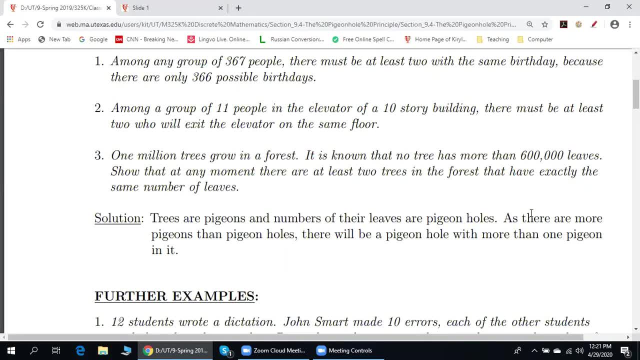 More than one pigeon in it Means at least two. Any questions about these three intra-level examples: When does it prove that there's three pigeons in a hole, Like does that work for that problem too? Well, here, at least two, not at least three. 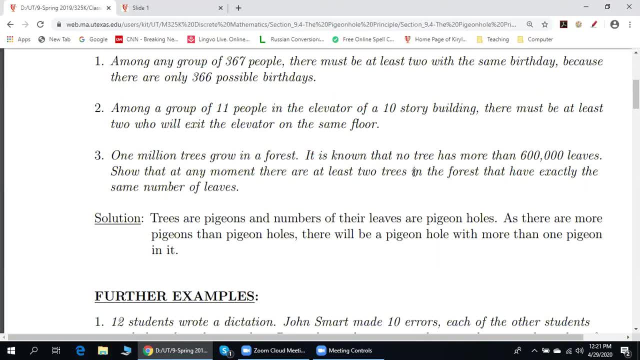 And why not? How would you say? Well, why not Think about the following? We think about the number of leaves as pigeonholes. How many pigeonholes do we have? 600,000.. 600,000.. Now, let us place into each pigeonhole first one pigeon, one tree. 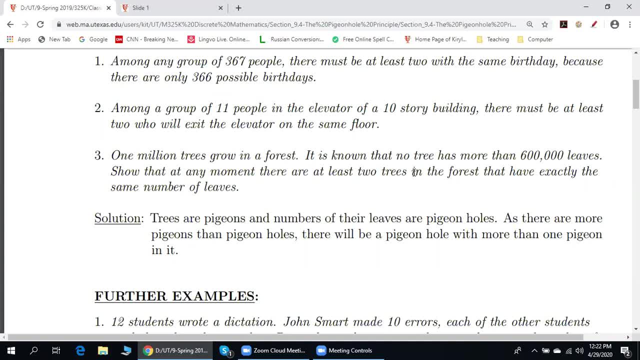 So 600,000 trees. The remaining number of trees is 400,000.. Now we place the remaining 400,000 trees into the same pigeonholes once again. In some pigeonholes there will be two trees, But since the total number of pigeonholes is 600,000,. 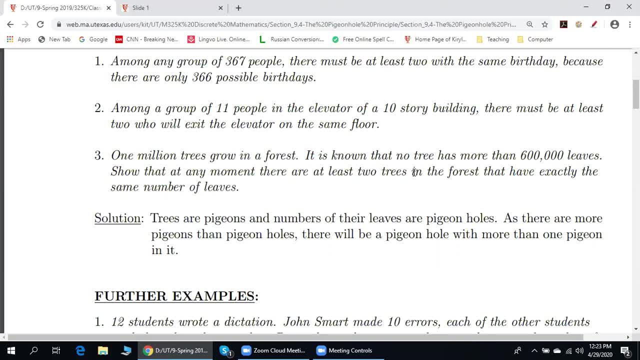 in some pigeonholes there will be two trees And the total number of remaining trees is 400,000.. There will be pigeonholes that have only one pigeon, So what number would it need to be for it to be three? For three pigeons it should be lesser than one half. 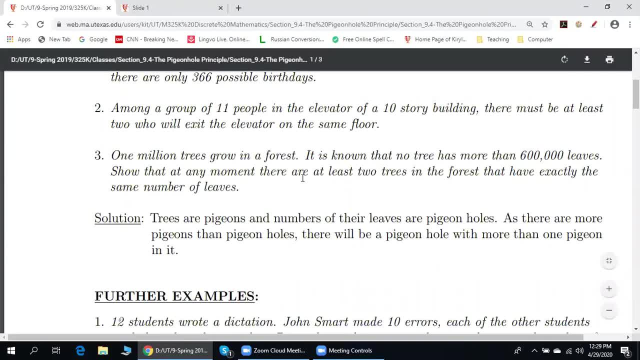 Yeah. To assure that, at any moment, there are at least two trees that have exactly the same number of leaves, We can replace this number by any number which is lesser than one million. To assure that there are at least three trees, we can replace this number by any number. 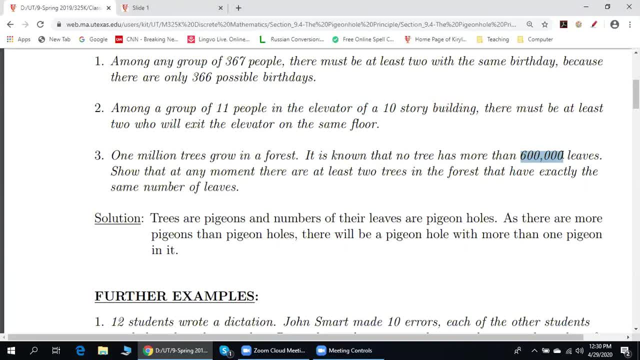 which is lesser than half, lesser than 500 million. Would a general pigeonhole principle be that KN plus one pigeons in N holes. so they'd have to have at least one hole with KN, Yeah, plus one pigeons, Yes. So if we want to replace two by k, we just divide one million by k minus. 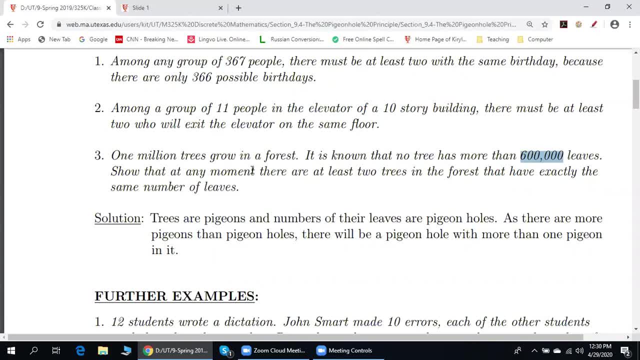 one. Okay, So this number should be less than one million divided by k minus one, For example. in our case k is two. We divide one million by two minus one by one, So we can replace this number by number which is lesser than one million. Any other questions here, Would that? 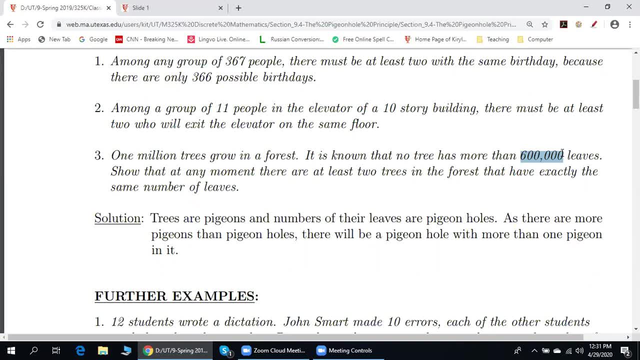 necessarily ensure that you would have at least k trees, or that just make it more likely Like it wouldn't. No, we are sure. We want to know for sure, Because, once again, if instead of 600,000, we put one million minus one, we still have more pigeons, which is one. 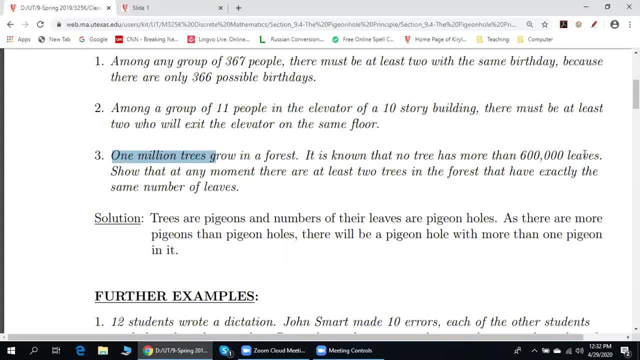 million than holes And we can apply the pigeonhole principle. This assures- we're not talking about probability- that if instead of 600,000, we put any number which is lesser than one million, then we- I see, I had an idea in my head and it was just wrong. Okay, thank you. 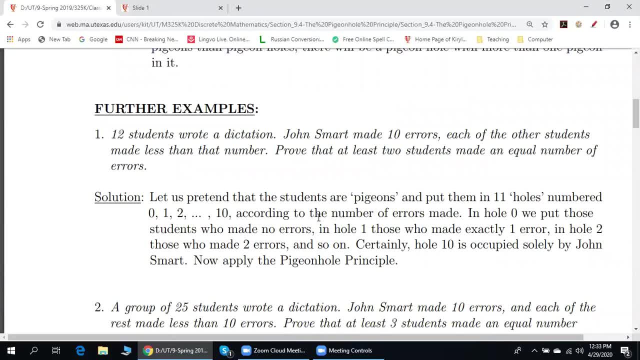 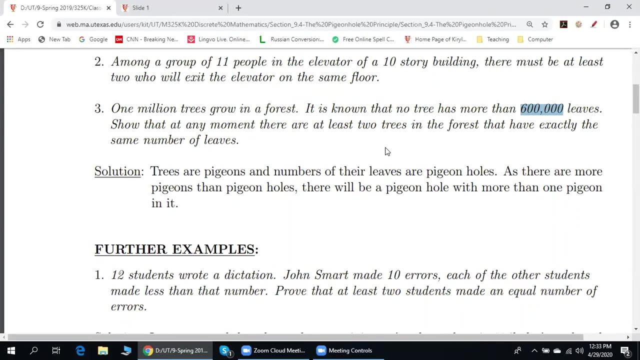 Next, Twelve students wrote a dictation. John Smart made 10 errors. Each of the other students made less than that number. Prove that at least two students made an error. Equal number of errors, Guys. how do we prove that? 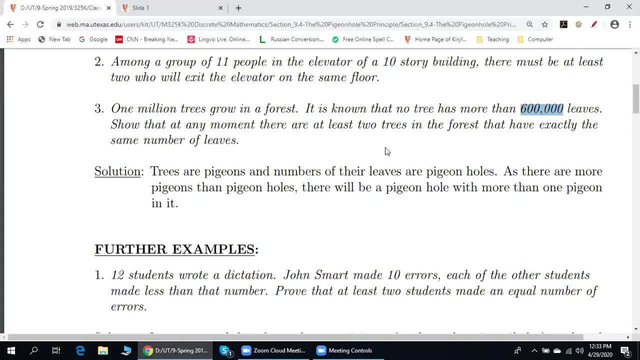 There are 12 students, and any student that makes less than 11 errors, then there must be at least two students that made less than 11 errors. So the maximum number of errors is 10.. We have 12 students in total. Our next question: 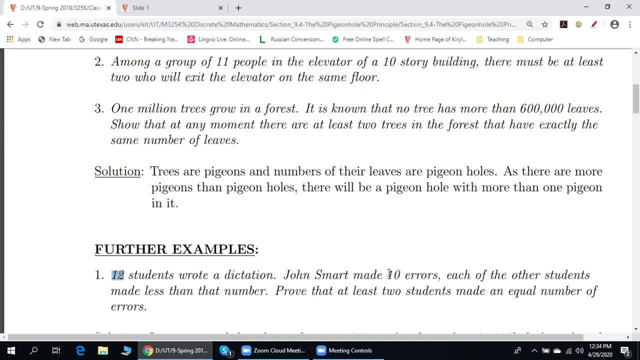 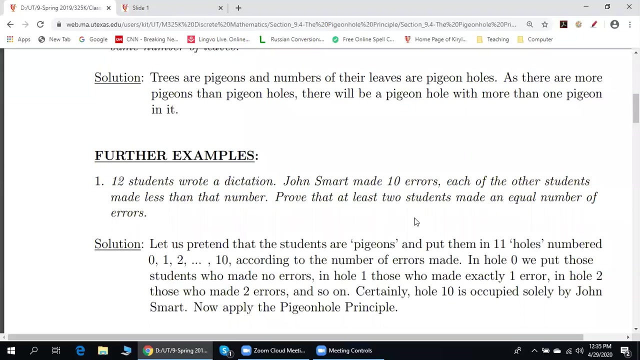 is one student made 10 errors. the remaining 11 students made 9 or lesser, So we have 11 students left. These students made either 9 errors or lesser. By the way, the number of possible errors is not 9 for the remaining 11 students, but 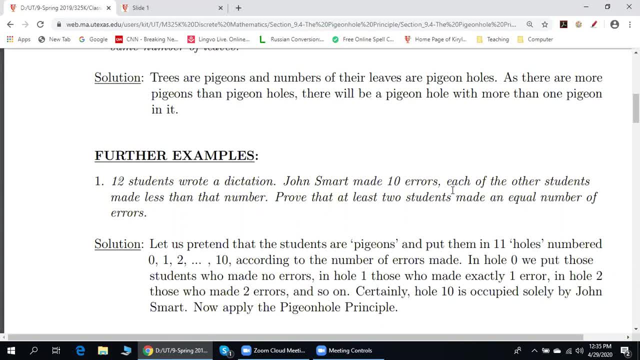 actually 10,, because it's from 0 to 9,. 10 possibilities. We have 10 possibilities for errors and we have 11 holes. We have more pigeons than holes. therefore, at least two students made an equal number of errors. 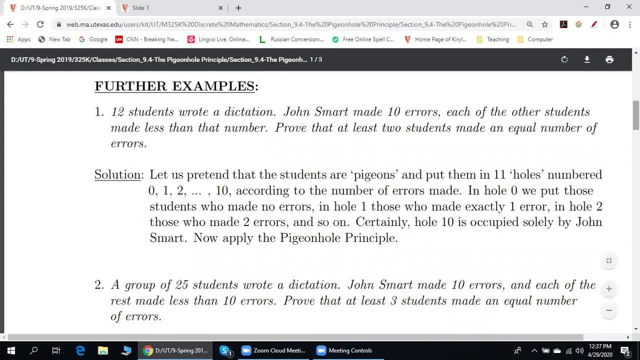 Here. a group of 25 students wrote a dictation. John Smart made 10 errors and each of the rest made a less than 10 errors proved that at least three students made an equal number of errors. How do we solve this problem? 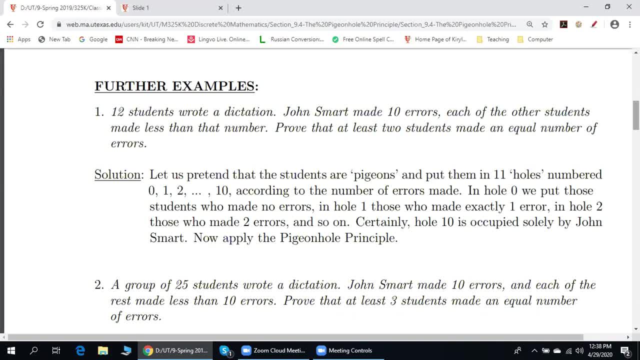 Do you show that 10 is less than 25 divided by 3 minus 1?? So let us think about it. The total number of students is 25.. But we exclude John Smart because the remaining 24 students made a lesser than 10 errors. 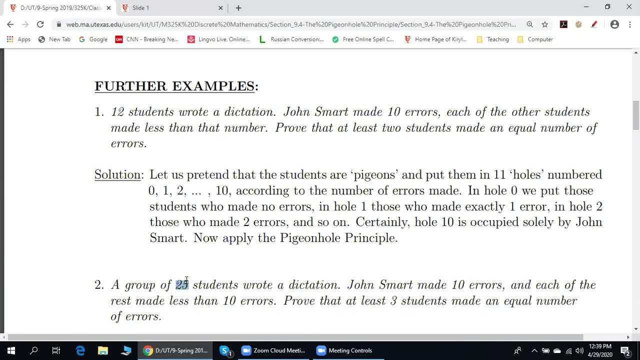 Correct. Yes, So the number of pigeon holes will be 10, because You're getting from 0 to 9, right From 0 to 9.. Absolutely, So we have 10 pigeon holes and 24 students. 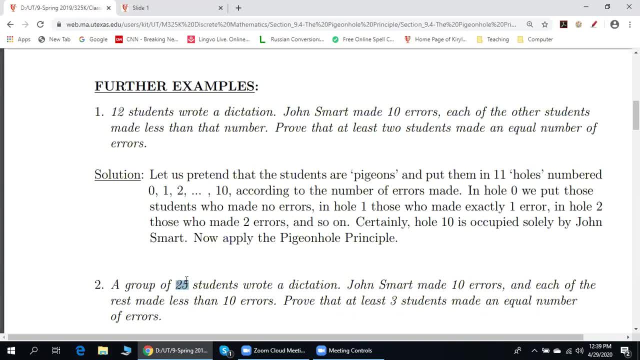 If we put 10 students into each pigeon hole, then 10 students again into each pigeon hole, In each pigeon hole there will be two students, but then we have four students left, which means there will be at least one pigeon hole with three or more students. 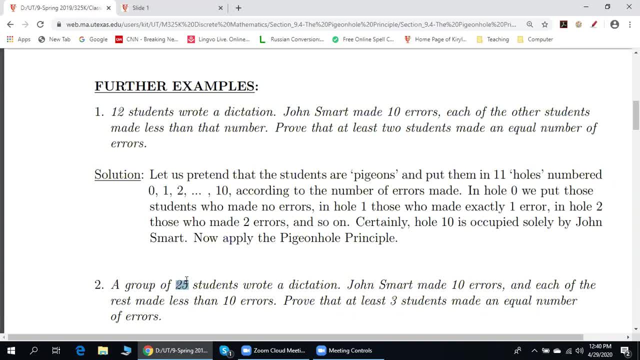 Any questions here? What if John Smart had made 13 errors here? So if we have 13 errors, then the rest made 12 or lesser. So we have 13 pigeon holes, 24 students. So we place first 13 students. 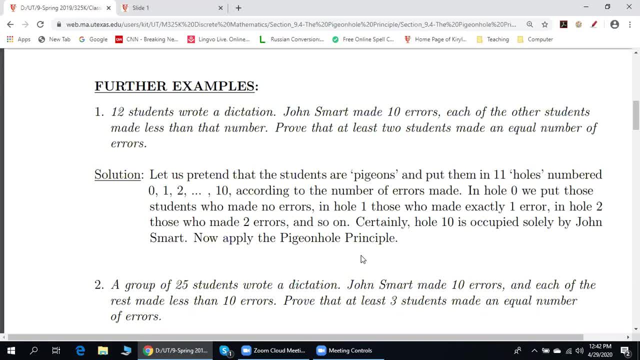 Then the remaining number of students will be 11.. Therefore, we cannot guarantee that there will be a pigeon hole with at least two pigeons. Does this answer your question? Yes, So if you replace 10 by 11, then we still can guarantee that there will be at least. 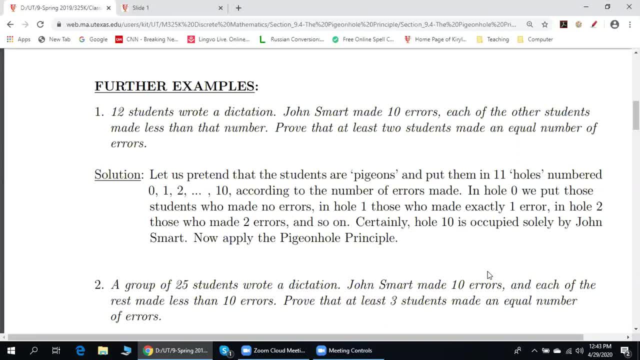 three students, But we cannot guarantee that there will be at least 3 students. But we cannot replace 10 by 12.. So, in order to ensure that at least 3 students made an equal number of errors, we can replace 10 by 11.. 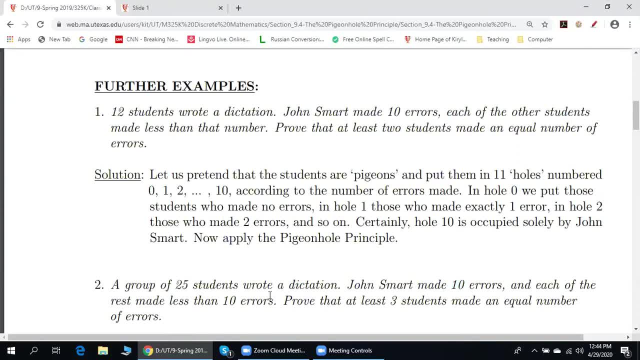 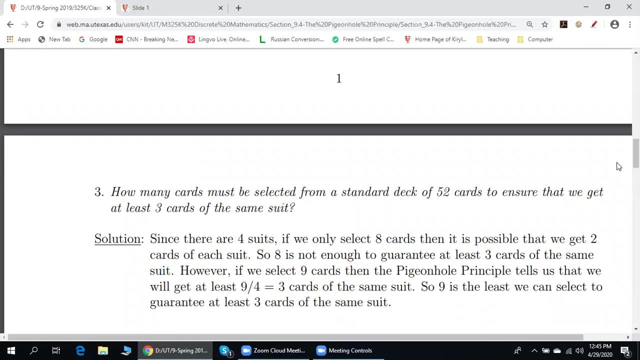 Here and here, But we cannot replace 10 by 12.. Here, How many cards must be selected from a standard deck of 52 cards to ensure that we get at least 3 cards. What do we do? First, you need to know that the suit is four.